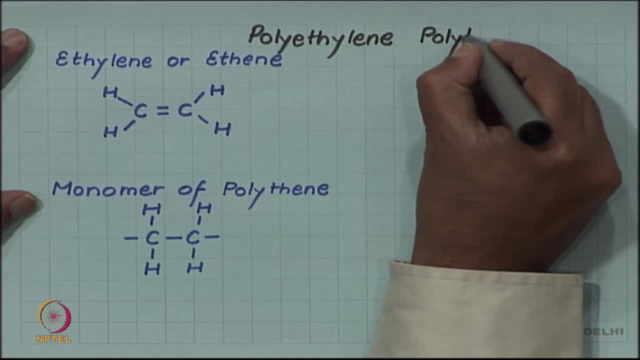 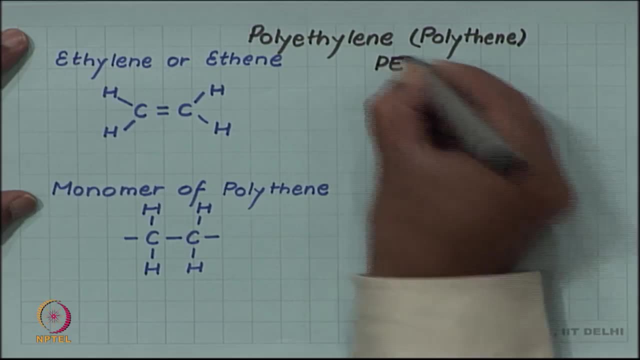 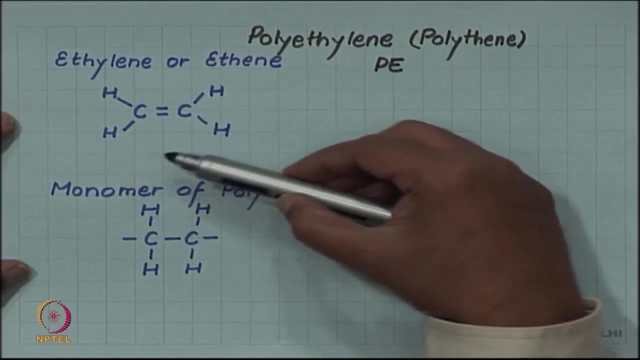 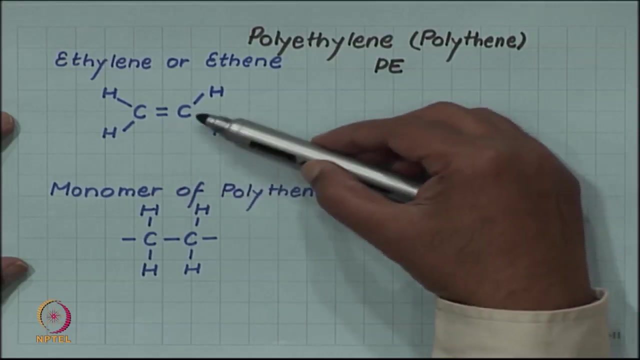 a risk factor for solutions. So these are complex, Therefore why we have to say it is aОs åf obten Challenge, also called polythene, abbreviated as PE. So this polymer is made of ethylene or ethene gas. In the gas you have a doubly bonded pair of carbon with two hydrogen attached to each of. 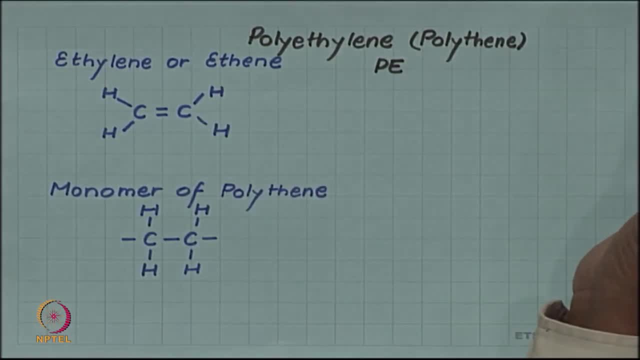 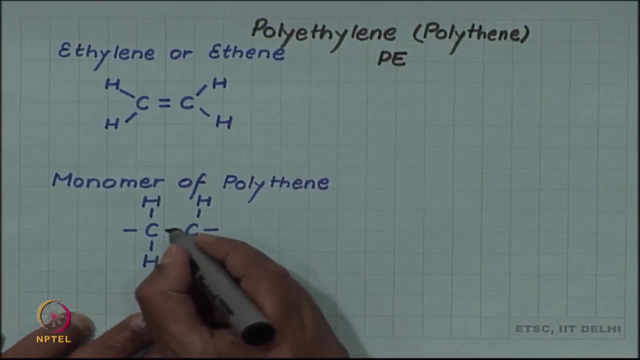 these carbon. but when this gas is polymerized, you get a monomer in which this double bond transforms now to a single bond, Thus satisfying the four bonds of carbon. you now have two free bonds which can join with other monomer or other molecules of ethylene. So this is 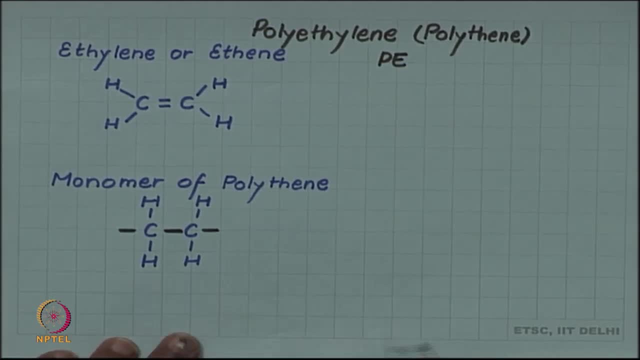 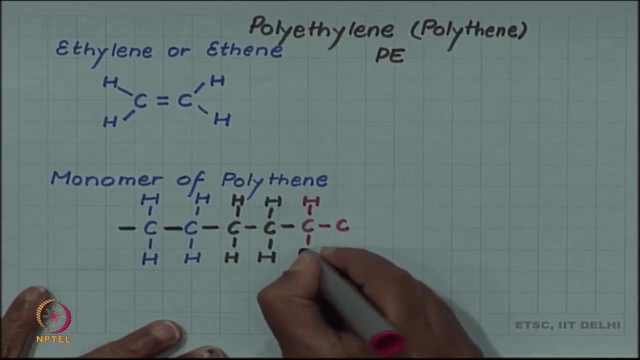 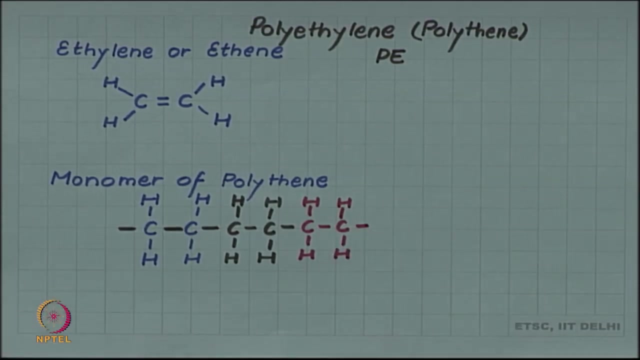 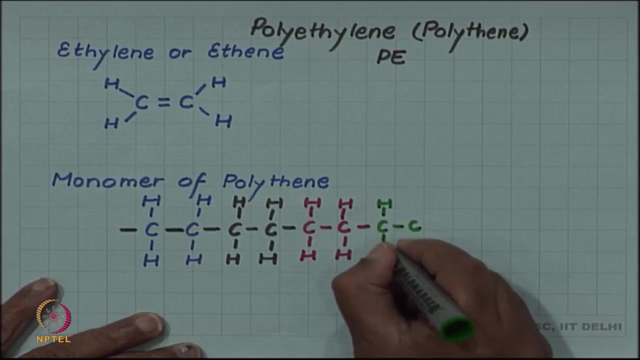 the basis of having long chain. Now, with the next carbon atom from a neighboring monomer, then what we have is we can say a dimer, Then yet another next third molecule can come and join with this. We have a trimer and if this process continues, you can see that you can have many, many monomers. 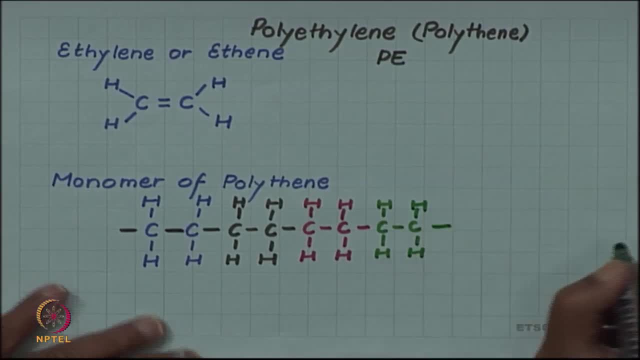 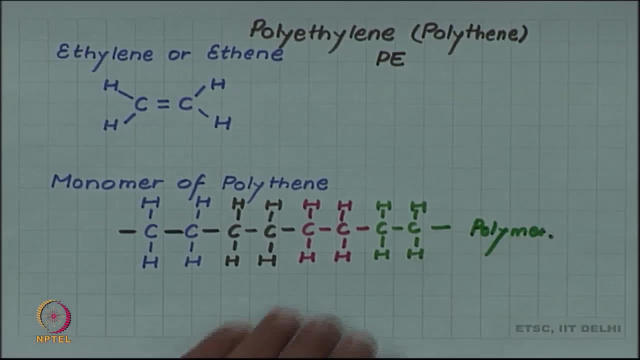 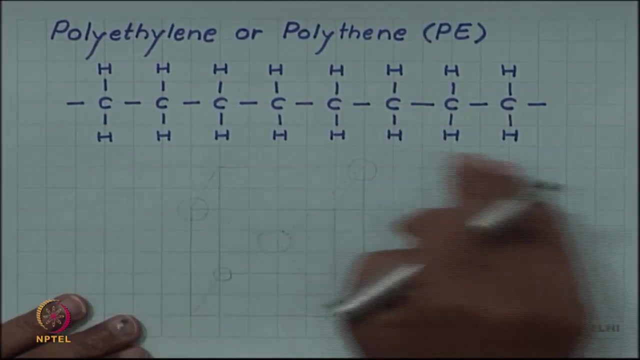 attached to single chain and that is what you have then a polymer. this will be a polymer. So polyethylene or polythene we have a single chain is a long chain molecule with many monomers, many monomers of each of the, each pair of. 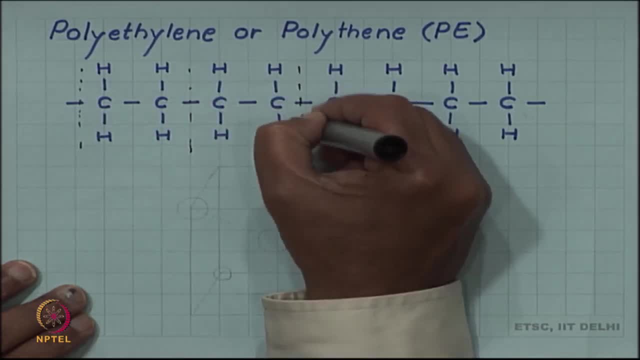 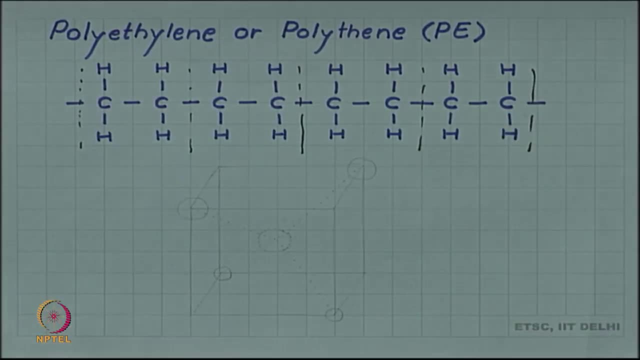 carbon atom is defining a monomer. So you have several monomers here which are connected to give you a macro molecule or a chain of polythene. I have drawn it here and I have drawn it in a planar way, which is a simple way of drawing, but one should recognize that. 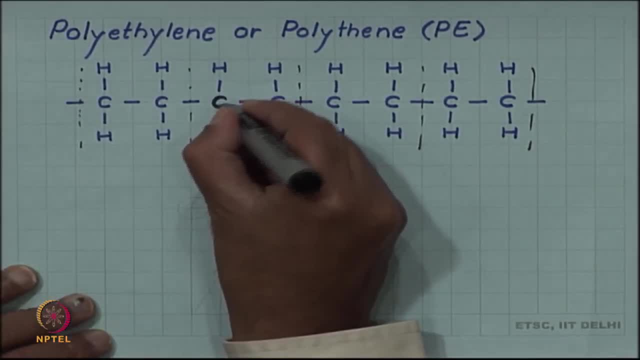 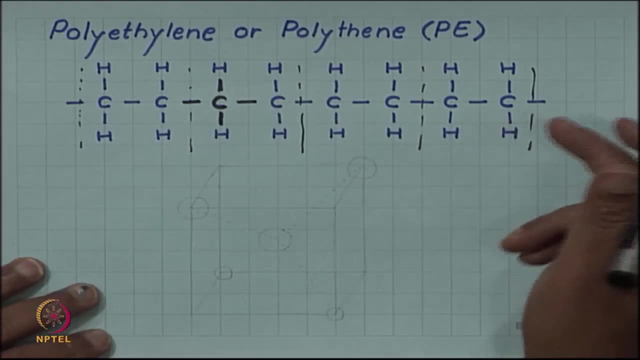 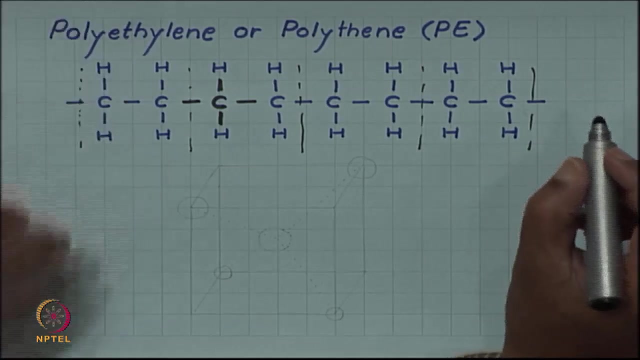 the bonds of carbon. if I take a single carbon, the four bonds of carbon are not in a plane. they are directed from vertices to the corners of a tetrahedron, So they are tetrahedral bonds. One way to think about these tetrahedral bonds is to place a carbon atom in the cube. 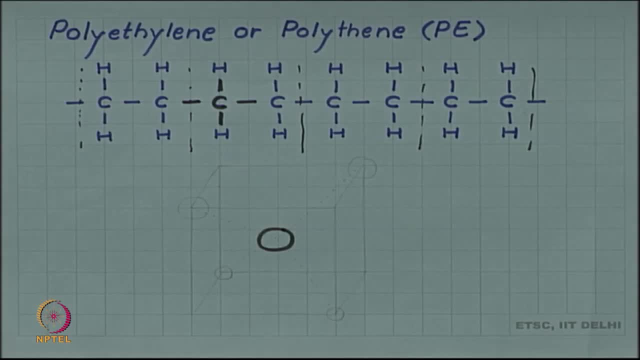 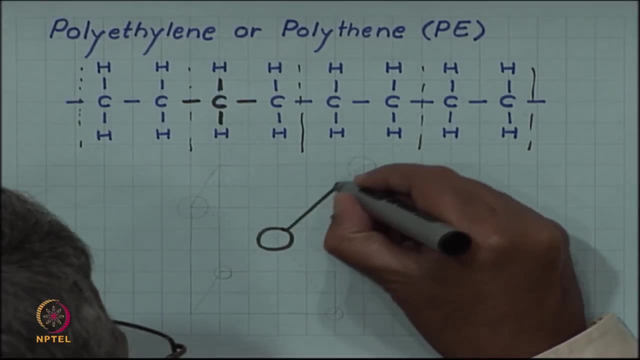 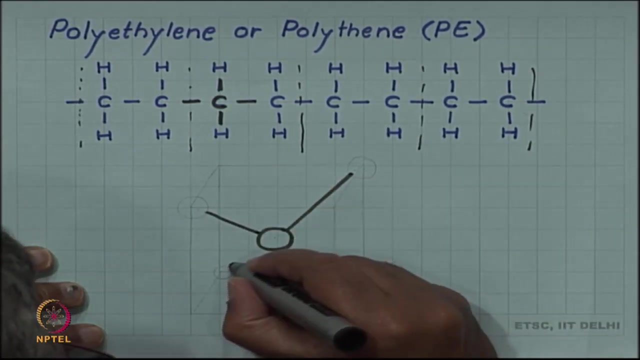 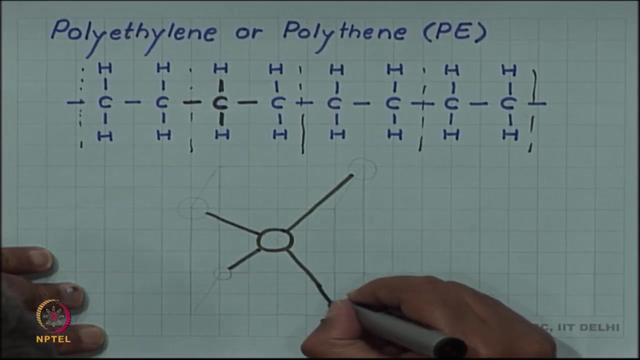 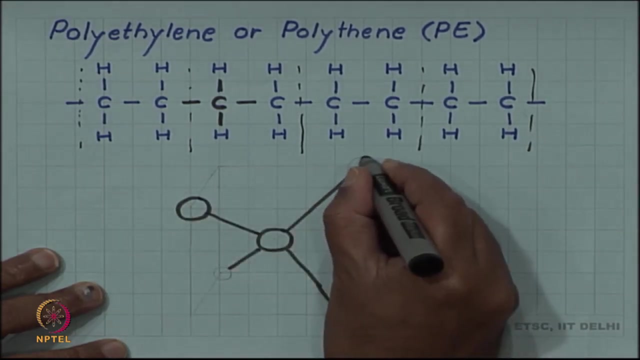 in the center of a cube and then draw these bonds as diagonals, body diagonals of the cube. So the two bonds are connected to carbon atoms. So I connect them to carbon atoms. 1 atoms and 2 are connected to hydrogen atoms. Let me show the hydrogen atoms in red. these 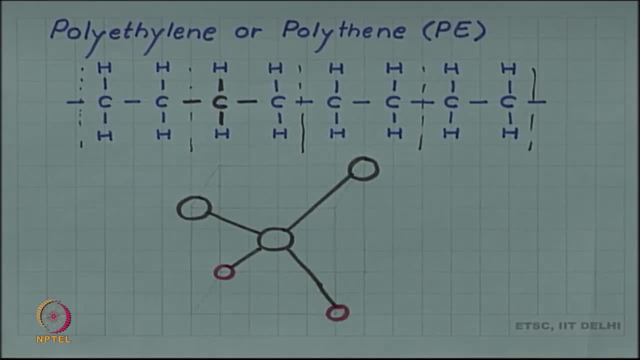 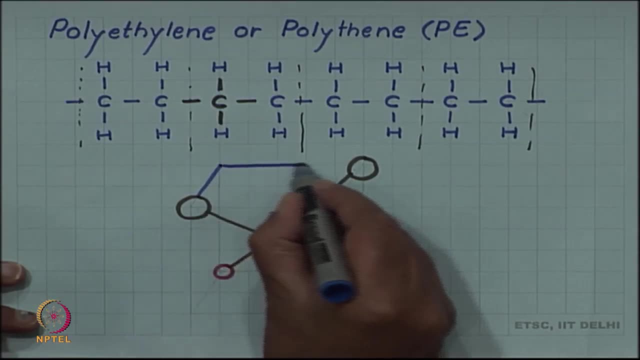 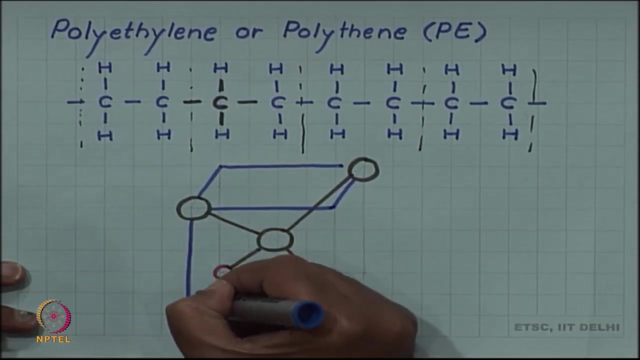 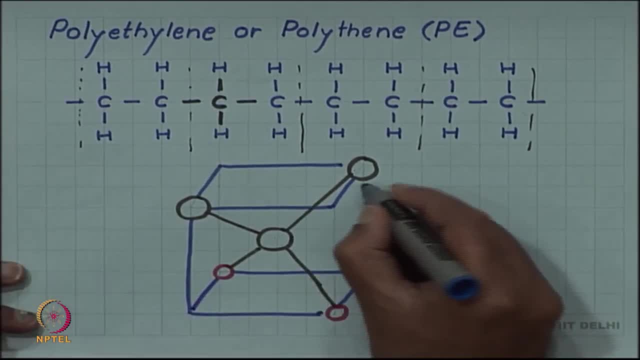 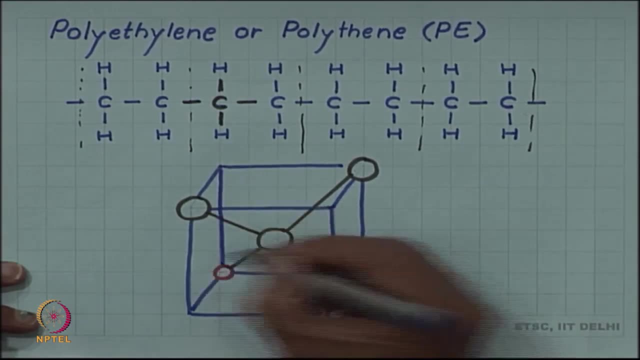 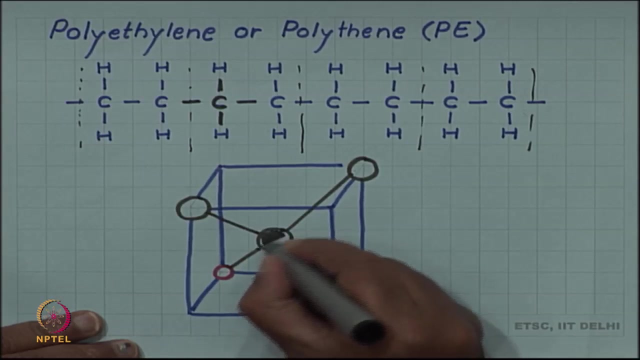 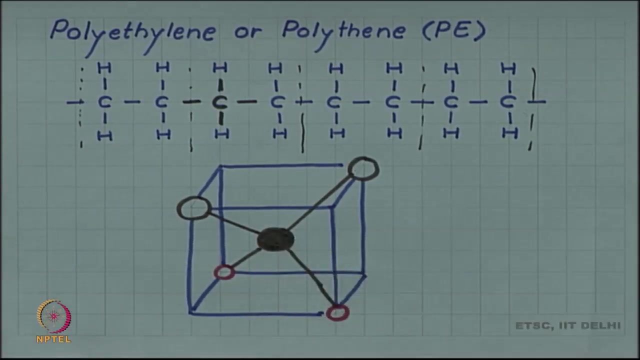 or you can say: alternating four corners of a cube define a tetrahedron. So if a central carbon atom which I now say dark- So this is the reference cube, this is the reference cube- has, it has its bond directed towards these corners and you have carbon at two of 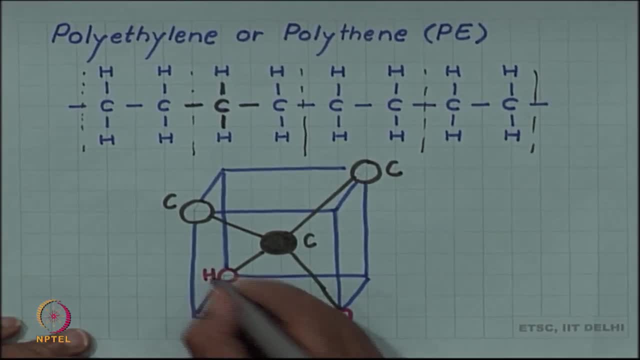 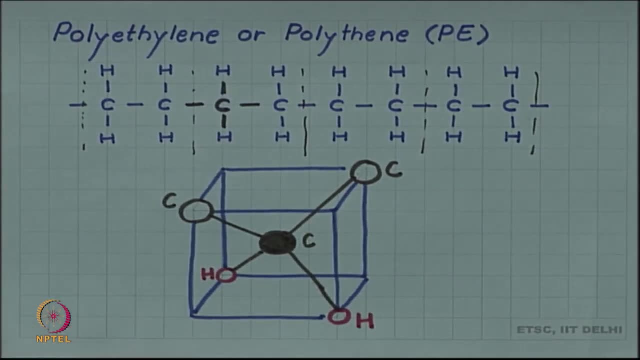 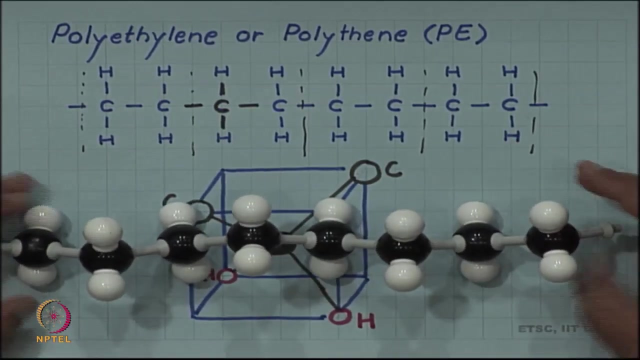 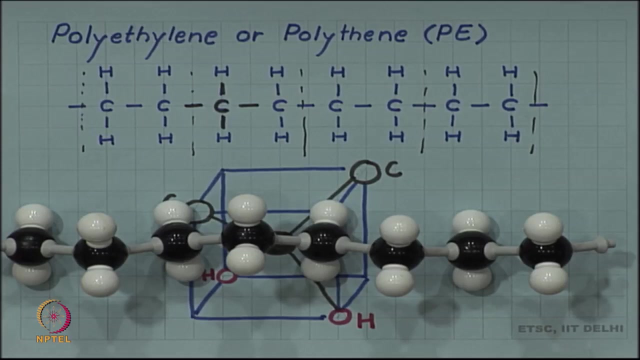 these corners and hydrogen at two others. So in reality, the this model is not planar but will have a three dimensional configuration. So here I have a 3 dimensional configuration molecule to show you. You can see, here we have 1,, 2,, 3, 4, 4 monomers are there and 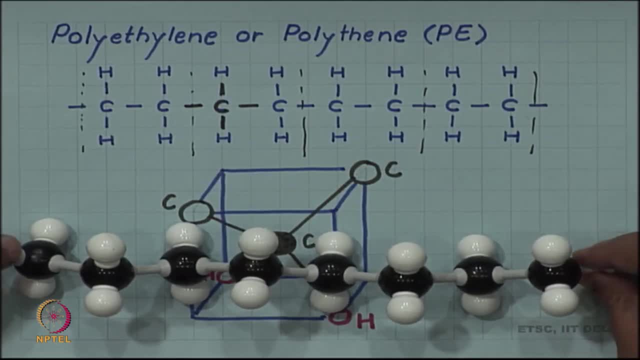 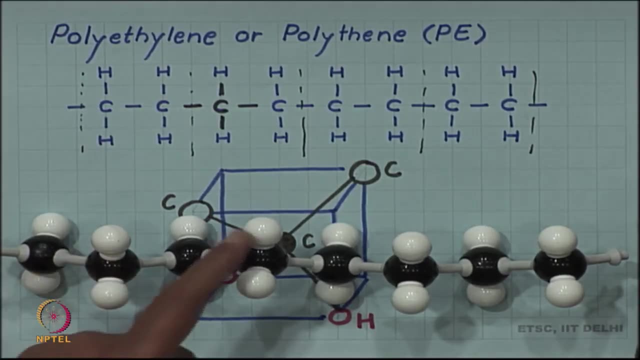 I have put them in a straightest possible configuration and we are looking from the top along this axis with the 2 hydrogen atom associated with each carbon. You can see that these 2 hydrogen atoms, the first 2 hydrogen atoms here, are on the downside of this chain. 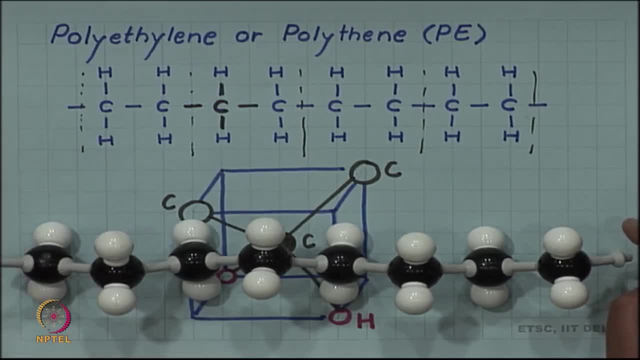 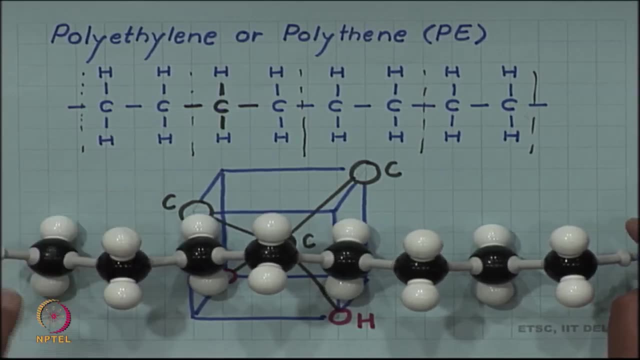 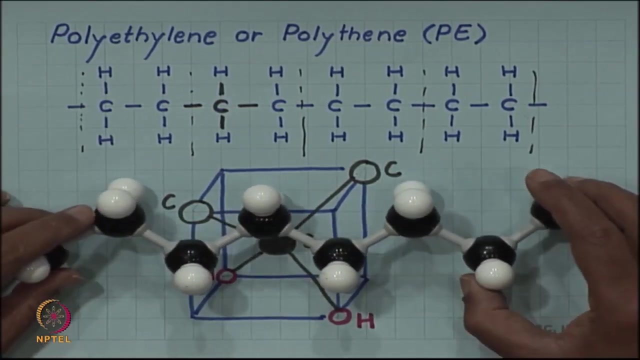 where as the other 2 are pointing up. So they are really not in the plane. they are pointing either down or up, depending upon the location of the carbon atom. The carbon atoms themselves are forming a zigzag formation, as shown here. So we are having a zigzag formation. 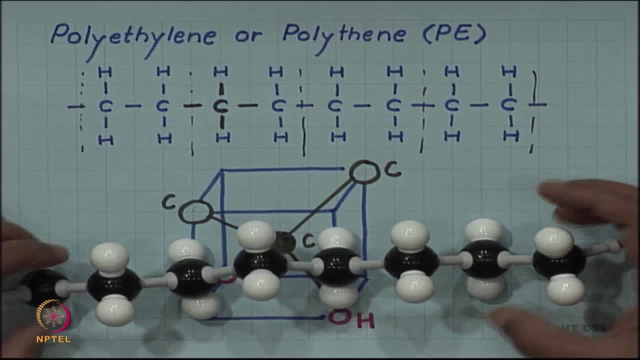 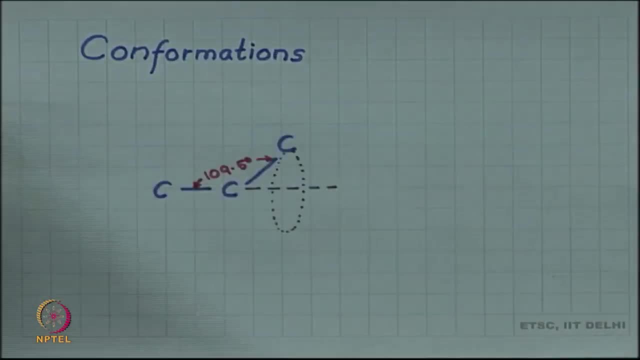 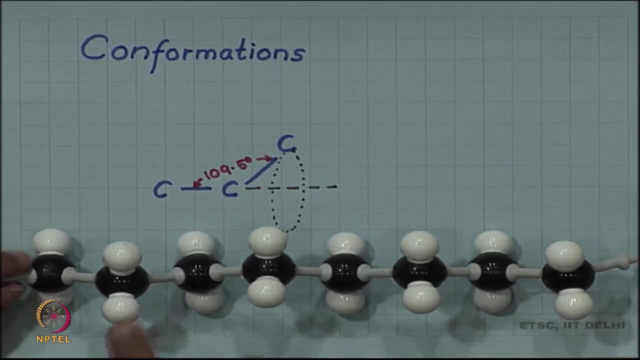 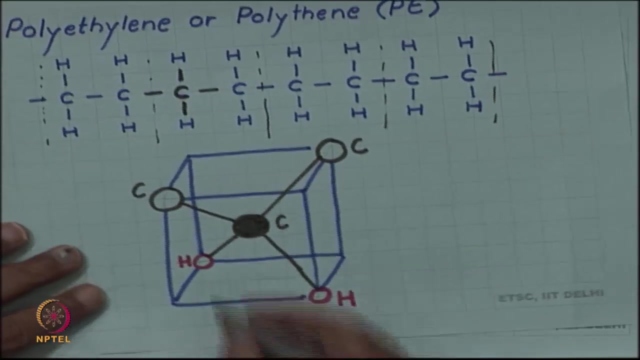 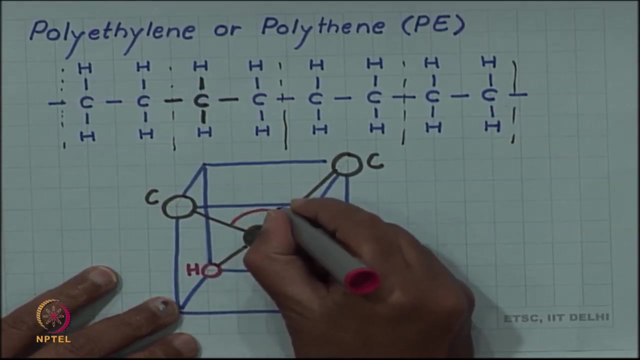 of carbon atoms. This is the straightest possible chain, this configuration for this chain. But the polymer, like this, has a degree of freedom of rotation about every bond keeping that angle. So this angle will be the tetrahedral angle of 109.5.. So that is the angle between. 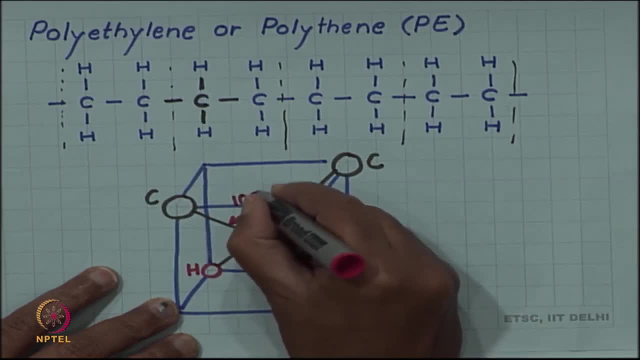 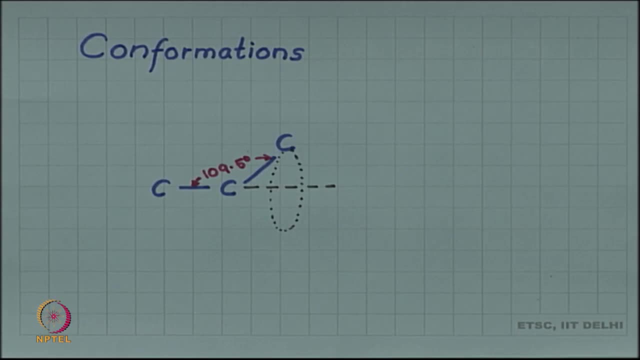 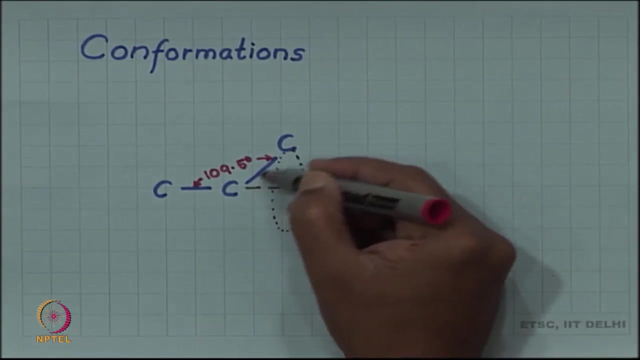 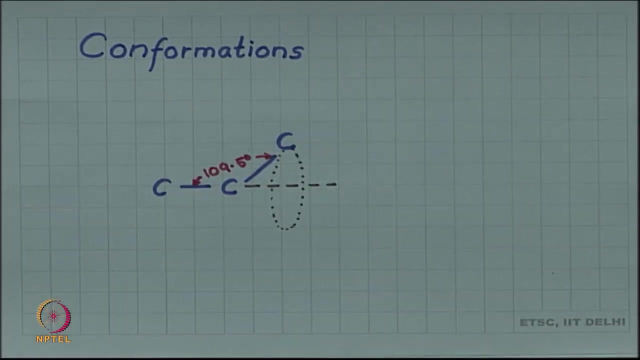 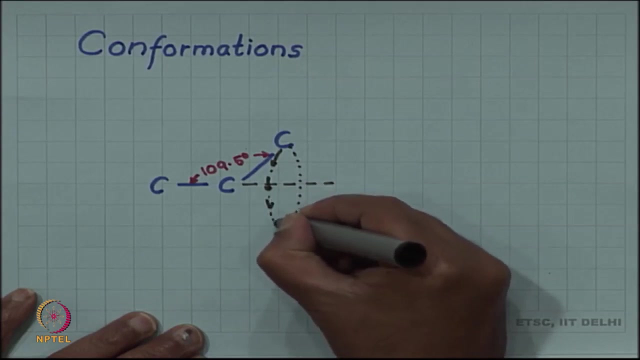 the body diagonals of a cube. So keeping this carbon, carbon bond angle as 109.5, there is possible to rotate any given bond about the other bond. So here I have shown that possible rotation. So I can take this carbon atom and I can rotate it in this manner about the. 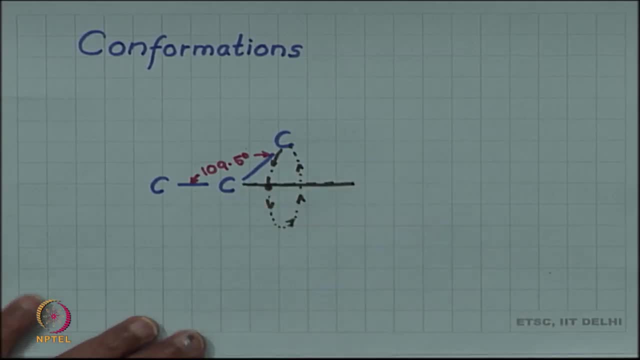 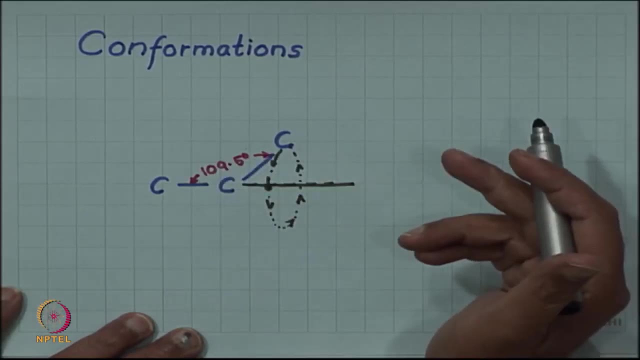 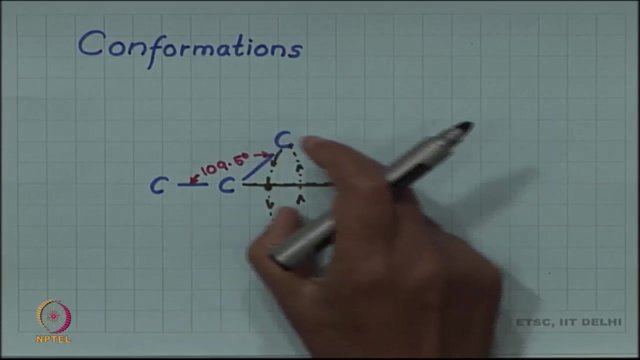 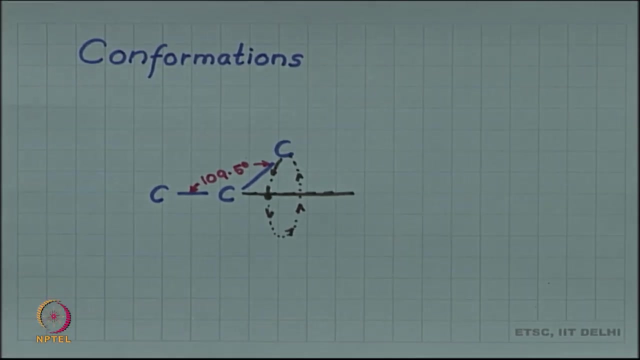 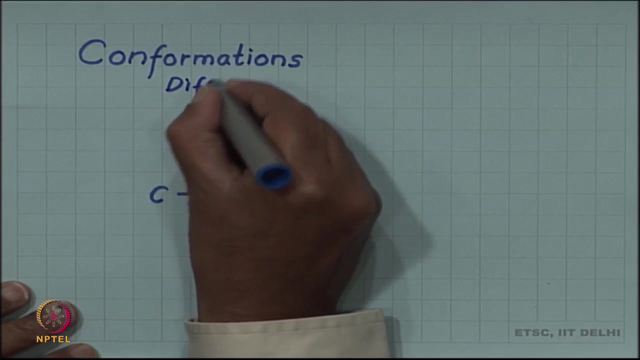 axis defined by the other bond. So if I rotate it about the axis defined by the other bond, this angle- 109.5 degree- will be preserved, But then the carbon-carbon structure will be taking different shapes in three dimensions. So these different shapes are called conformations. So conformations are different shapes different. 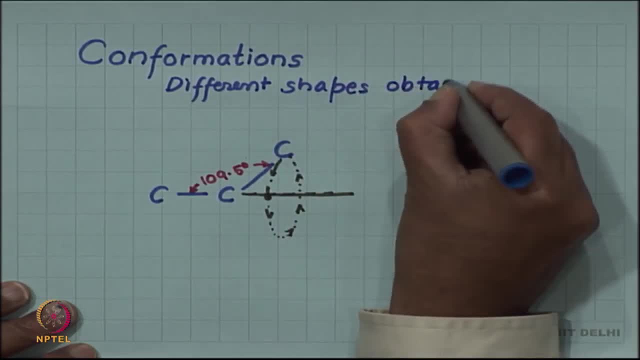 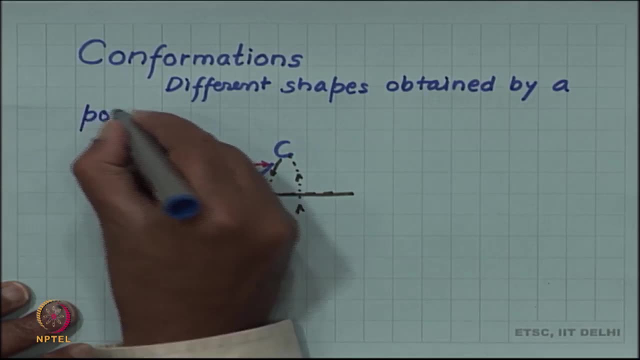 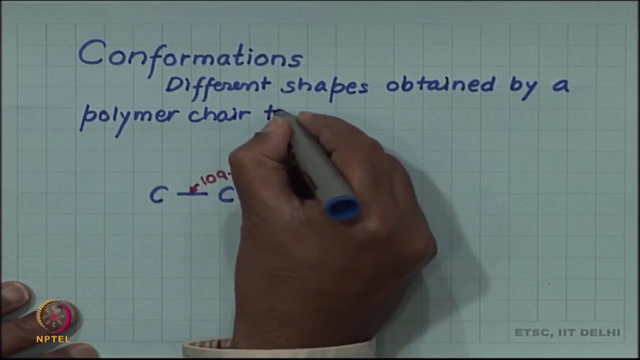 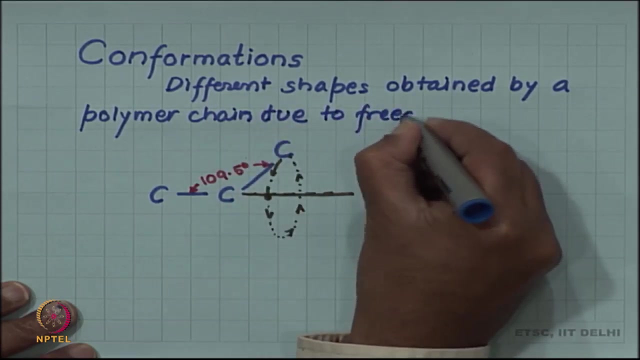 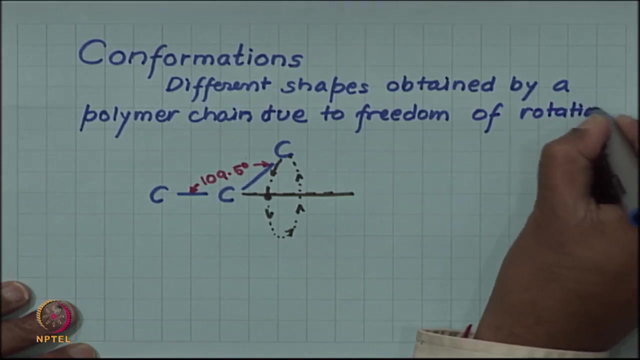 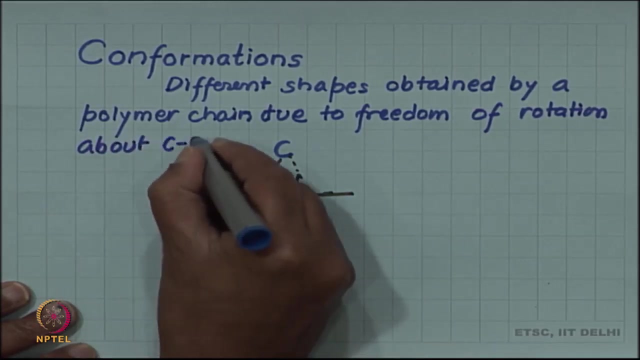 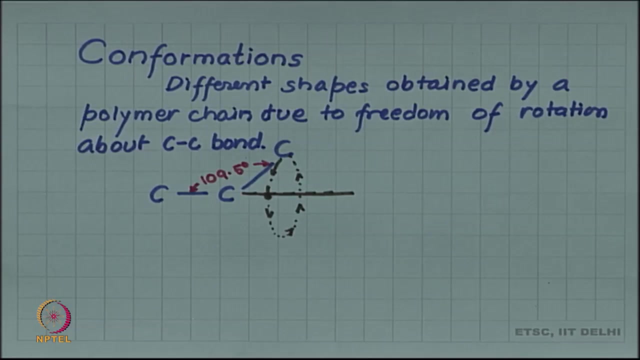 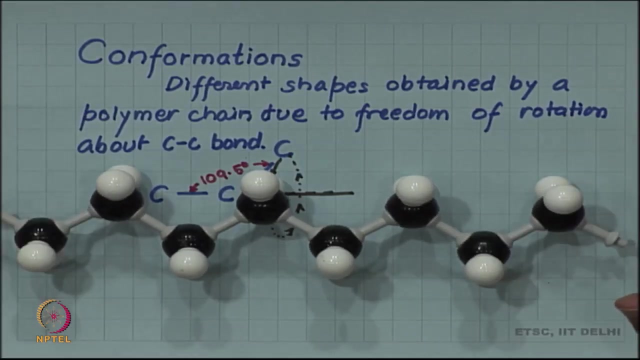 shapes obtained by a polymer chain. Polymer chain due to freedom of rotation about carbon-carbon bond. We can see this from again from our molecule here. So this is a very straight chain. although it is zigzag, this is the straightest possible. Why I am. 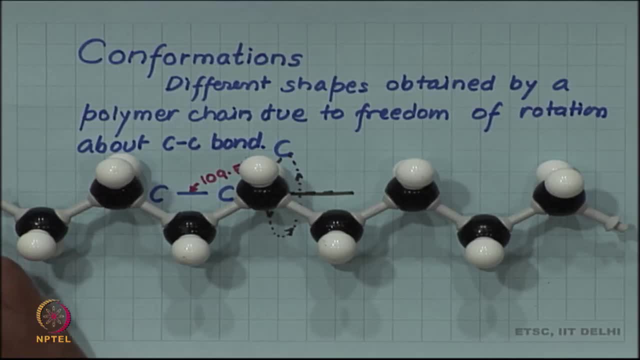 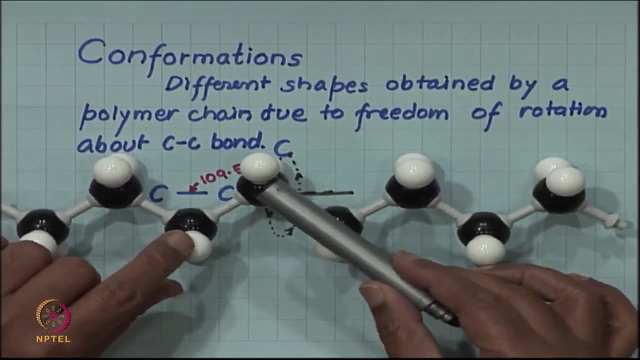 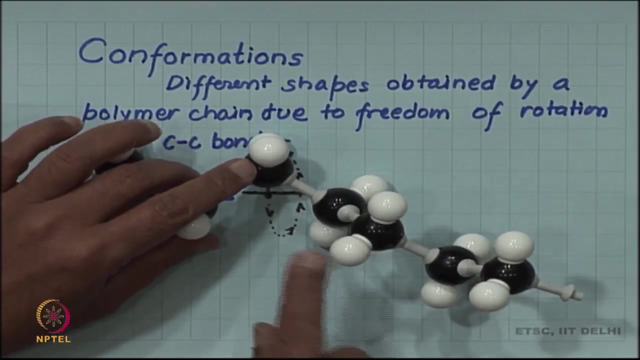 saying this, That there is a freedom of rotation about every bond. So let me use that freedom and start rotating. So let us say I am rotating about this bond, about this bond. So if I start rotating about this bond, I can flip this segment of the molecule out of the plane. 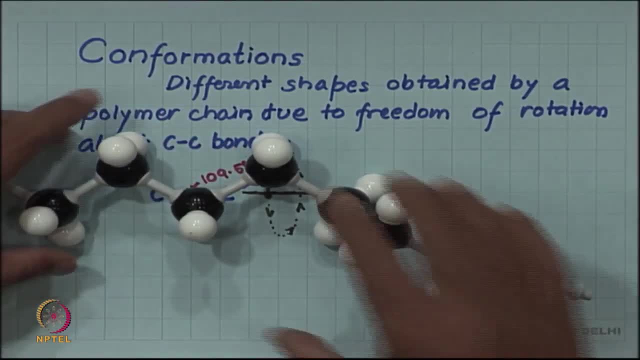 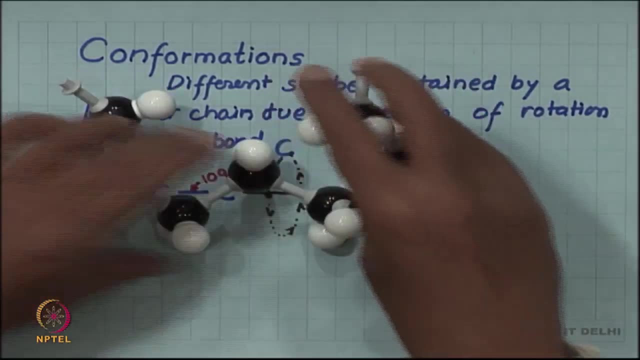 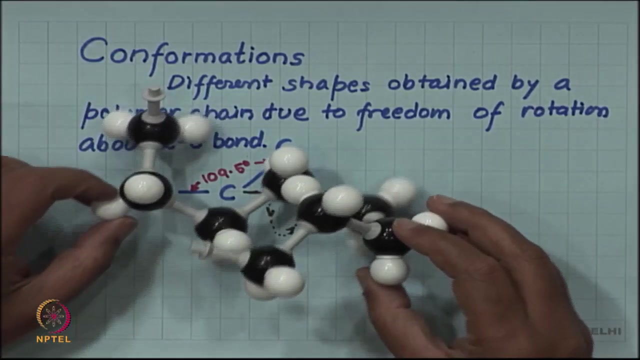 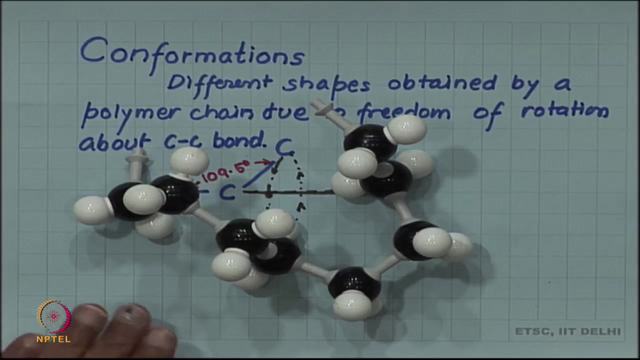 of the paper. So, and if I keep using rotations about other bond, So I can have a freedom of rotation, a molecule which is no more straight and is going in three dimension in a different conformation. So this is different conformation, So what I have is the same. 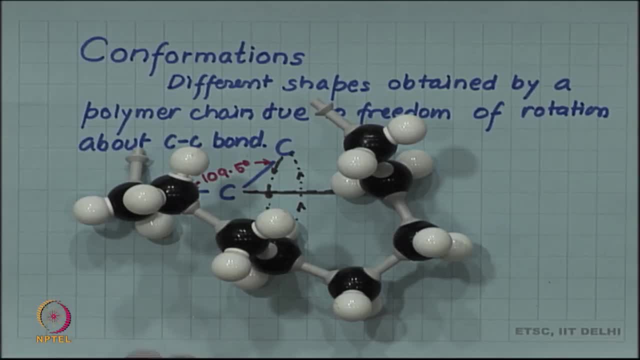 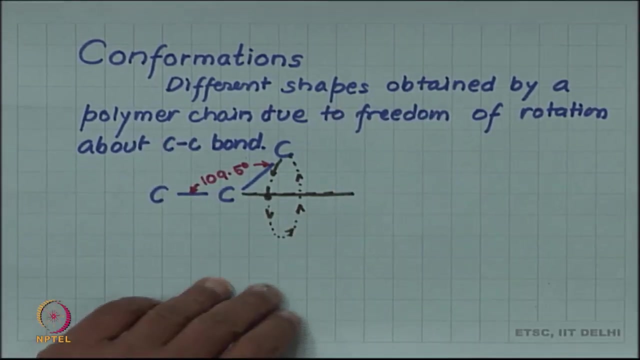 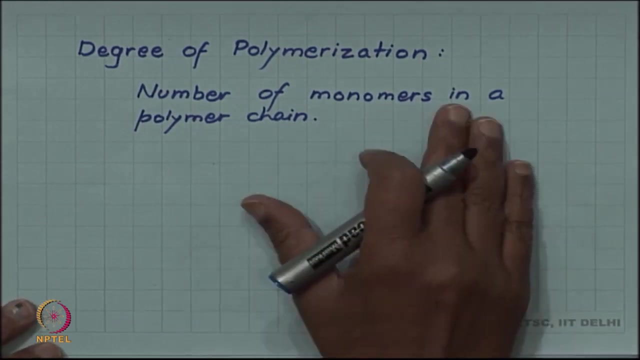 molecule, but in a different conformation, Each bond angle. if one carefully looks at each bond angle, is still 109.5.. The shape of the molecule in the three dimension is very, very different from the straight chain I started with. There is also a term, degree of polymerization, which is number of monomers. 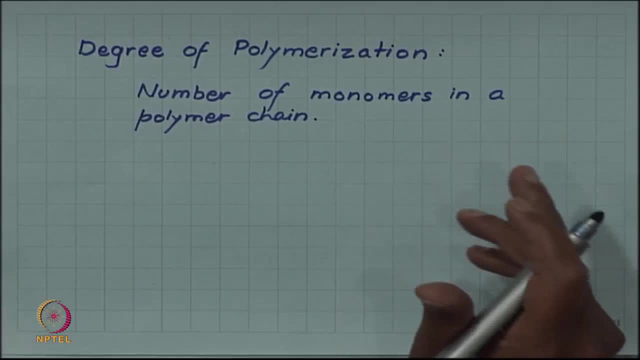 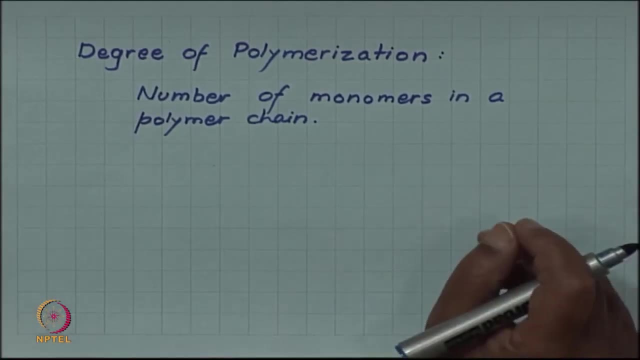 in a polymer chain. This tells us how long the polymer age. Many of the properties of polymer depends upon the length of the polymer chain, or the degree of polymerization. So of course, every chain, every single chain, will have a degree of polymerization. And degree of polymerization of a polymer sample will be an average of that degree of polymerization of different chains within that polymer. A macro molecule was originally proposed by Hermann St Alonger in about 1920..